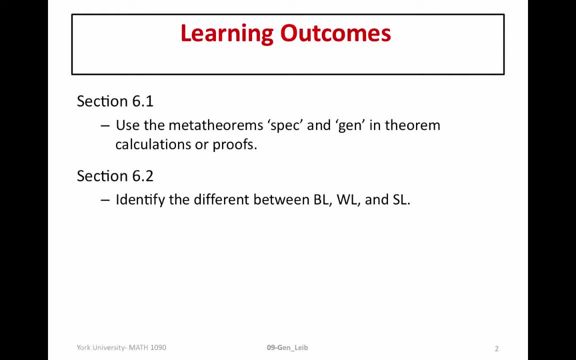 in our Hilbert proofs, And then we'll cover section 6.2, and within this section you'll be able to identify the difference between BL, WL and SL. SL, which stand for Boolean Labneh's, which is our rule of inference, weak Labneh's, which 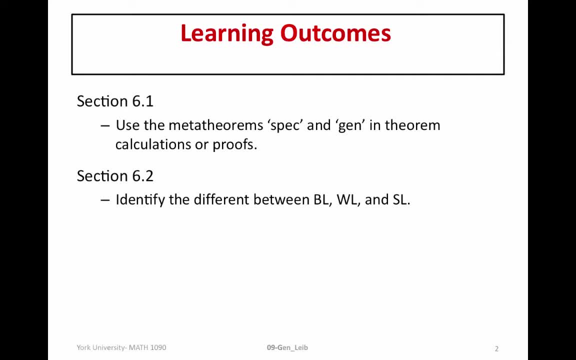 will learn what that is and strong Labneh's, and we'll also learn what that is, And then you'll also be able to use both weak Labneh's and strong Labneh's in theorem calculations or proofs in predicate logic, And these are going to be most helpful in equation style. 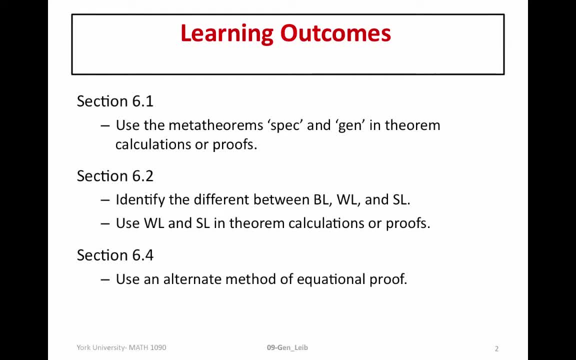 proofs. We will also cover section 6.4 in class, which is the proofs in predicate logic. So we're going to cover section 6.4 in class, which is essentially to use an alternate method of the equation proof. So we will use the 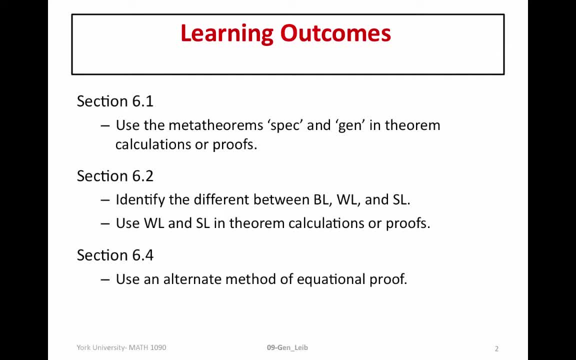 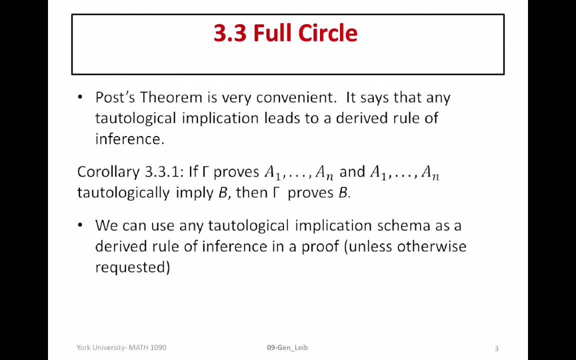 same equation style proof as we did before, but we're also going to introduce an alternate method to help us to write other kinds of proofs in predicate logic. Okay, so now that we are getting into theorem calculations or writing Hilbert and equation style proofs in predicate logic, we need to review a few things that we can use. 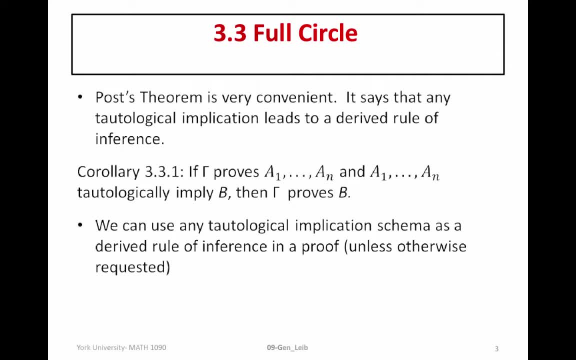 So recall, when we studied Poe's theorem, which is the completeness of Boolean or propositional logic, we discovered that Poe's theorem allows us to simply use any tautological implications as derived rules of inference. So instead of having to prove some kind of relative theorem, 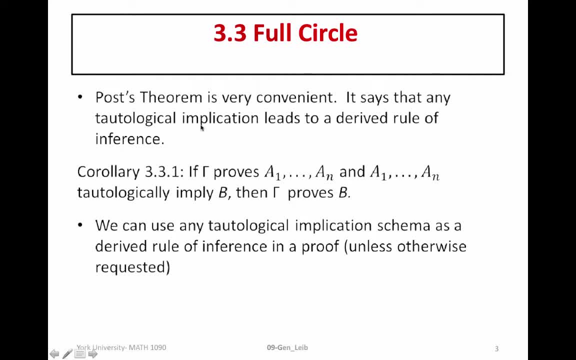 to be able to use it. we could just simply justify through tautological implication the use of truth tables, And this is a relative theorem or derived rule of inference that we can apply within our proofs. And this corollary simply formalizes that statement. So it says that if gamma proves, 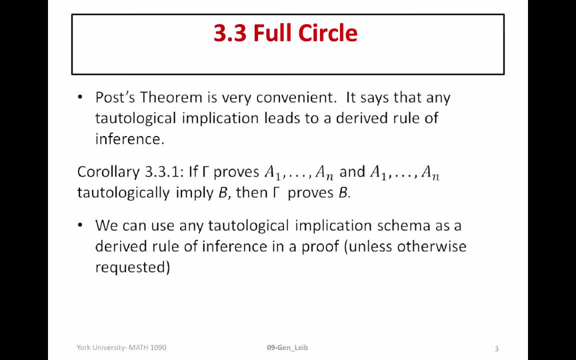 well-formed formula: A1 through An and A1 through An tautologically imply B, then gamma proves B. So essentially, if we have any of these statements written in our Hilbert proof and we can use all of these assumptions and know that they tautologically imply B, then 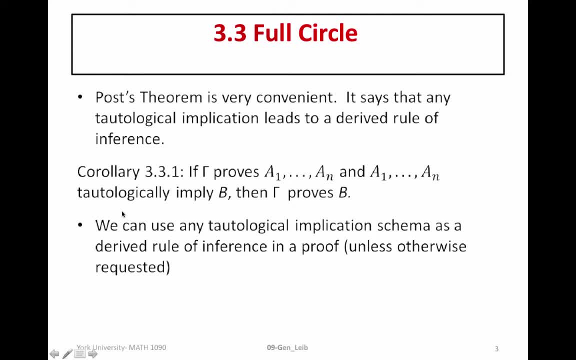 we can use this completeness, or Poe's theorem, or tautological implication, all of those different annotations, to be able to write B within our Hilbert proof. So essentially, to summarize, we can use any tautological implication schema as a derived. 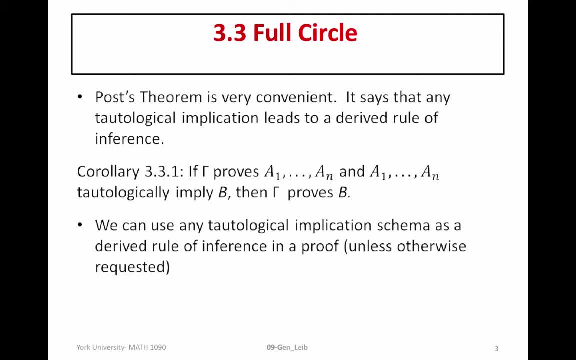 rule of inference in our proofs And that we did at the end of the course. Thank you, The first half of the course in propositional logic. So on the midterm, for example, you were able to use truth table arguments on the side of your page to be able to incorporate. 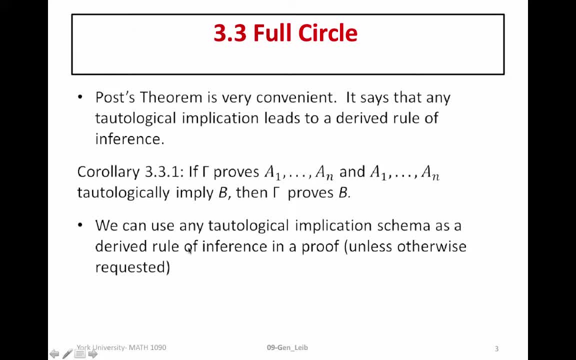 into your proofs, Or you were able to use truth table arguments entirely to prove something as well. We need to be a little bit careful as we move into predicate logic and using tautological implications. So, for example, we do not know that predicate logic is complete, So we don't have this same understanding. 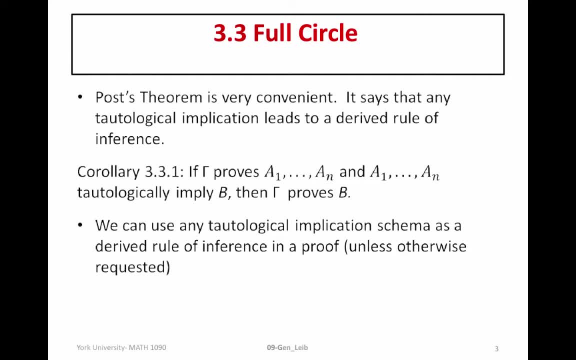 of completeness within predicate logic just yet, And we'll discover at the end of the course that it's both complete and incomplete at the same time, And we'll go through what I mean by that. But we can use Poe's theorem, which is why we're using this terminology, recalling that 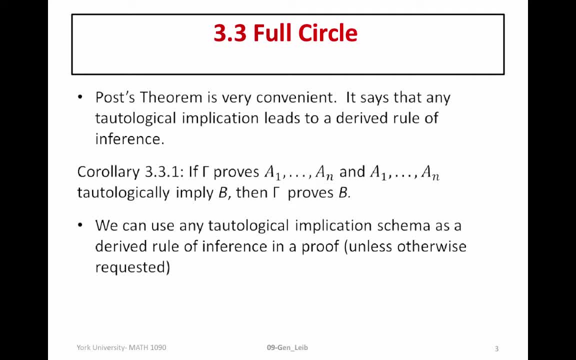 from last class implication within predicate logic is simply taking the abstraction of a well-formed formula in predicate logic and defining tautological implication in the same way as for propositional logic. So we're going to be able to use tautological implication or post theorem in our proofs and 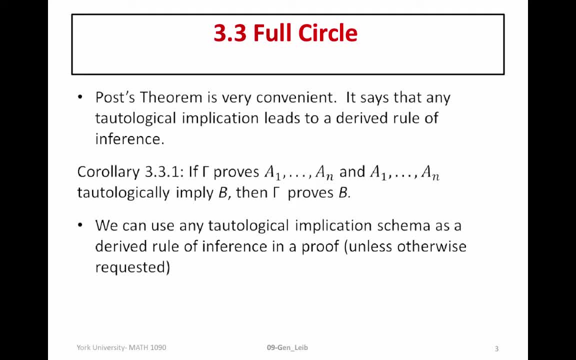 predicate logic, so long as we're only concentrating on the actions of the connectives and not worried about any of the new non-Boolean symbols that we've added. So we'll see examples of this later on, but the one thing I want to draw your attention to here is that, as you look through proofs within, 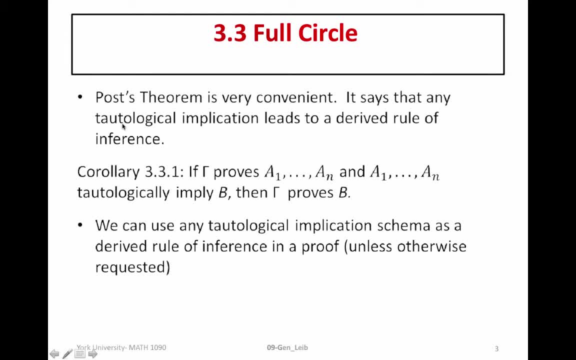 the textbook. for example, oftentimes the annotation is going to identify tautological implication. So this means that they've applied post theorem on simply the connectives by abstracting the rest of the connectives, And we can look at an example of this in class for sure. So that's. 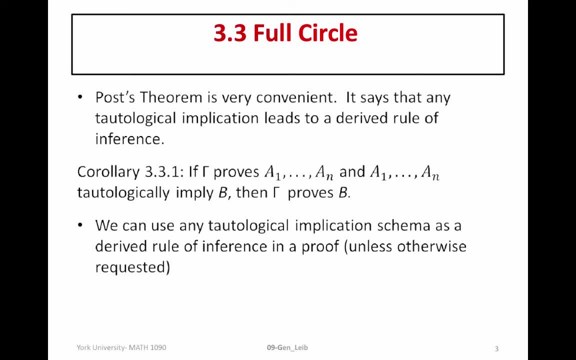 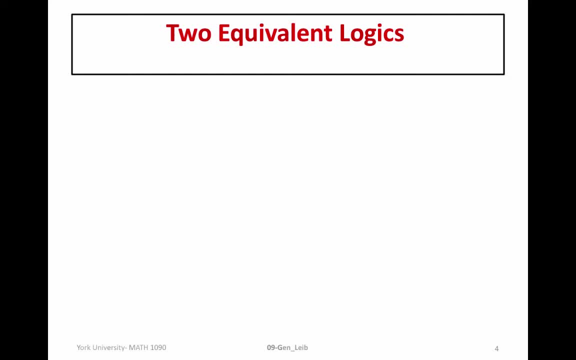 one thing that I want to draw your attention to in terms of proofs within predicate logic. The other thing that we've talked about is this notion of equivalent logics. So what do I mean by that? So two different logics are equivalent if, and only if. 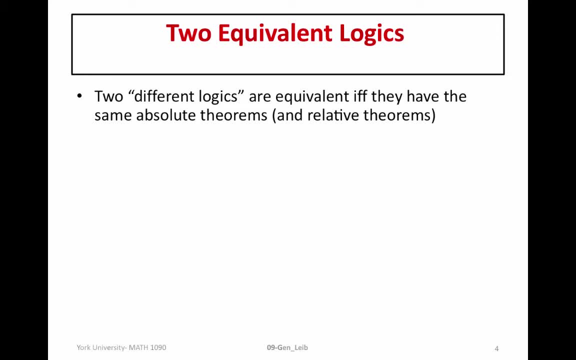 they have the same absolute theorems and relative theorems. So we talked about this a little bit when we were comparing the logic we defined, in particular Boolean logic, with the logic that you're kind of used to in Math 1090. And we talked about one of the first rules you learned in 1019, one of those main rules. 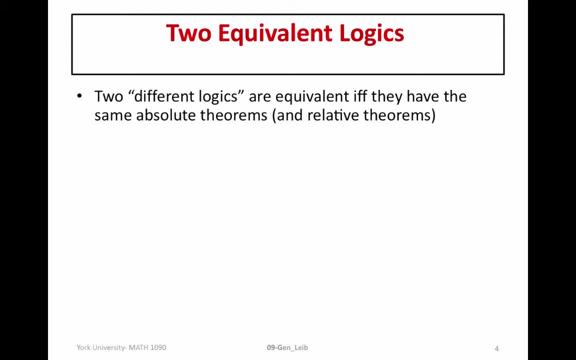 that you recognize was modus ponens, And I think I mentioned to you in class that it turns out that it is equivalent to define our logic the way we did with the two rules of inference, Equian and Labnese, and to define it using only modus ponens. So we can prove. 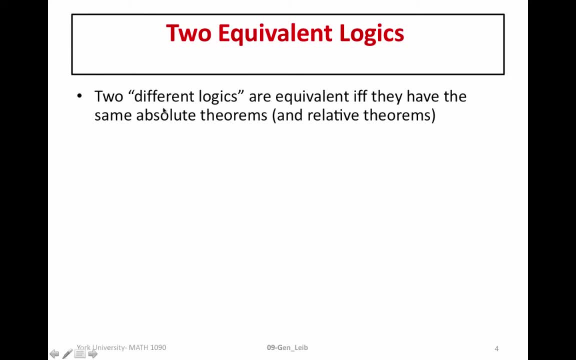 and it is proved in chapter 5, that these two different logics will have the same absolute theorems and relative theorems, and so they are equivalent. So let's represent logic 1 by our now predicate logic with primary rules- Equian and Boolean Labnese- And let's let logic 2 be predicate logic with one primary. 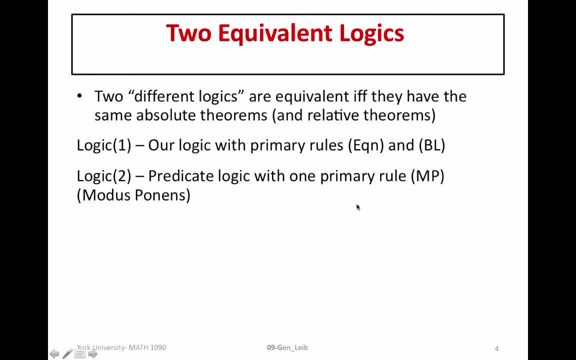 rule modus ponens right. So this is that if we have A and if we know that A implies B, then we can conclude B right. So that's what the modus ponens rule of inference says. So using a couple of lemmas, we can show- and it is shown in chapter 5, that these two 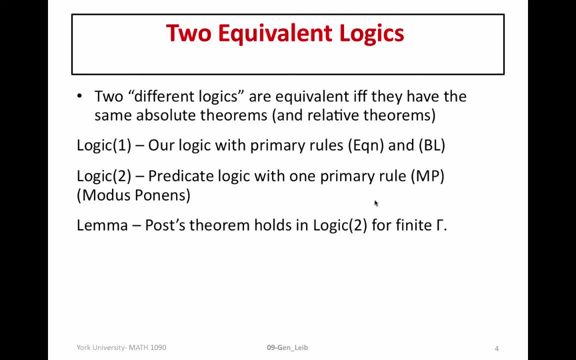 logics are in fact equivalent. So the first lemma says that post-theorem holds in logic 2 for finite gamma. So here we call: post-theorem is the completeness of propositional logic. So here we're only looking at the definition of tautological implication, focusing on simply. 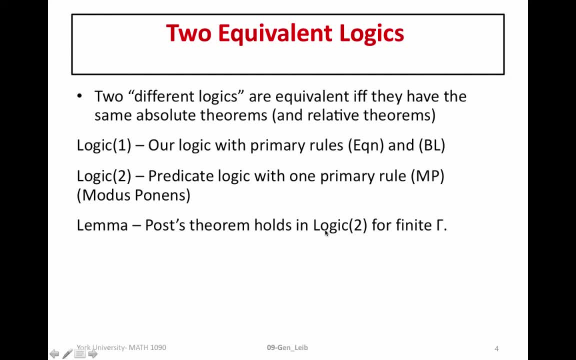 the connectives, getting rid of any non-Boolean symbols. So we can prove- I'm using modus ponens- that post-theorem holds. And then you can also prove that logic 2 has Equian and Boolean Labnese as derived rules.